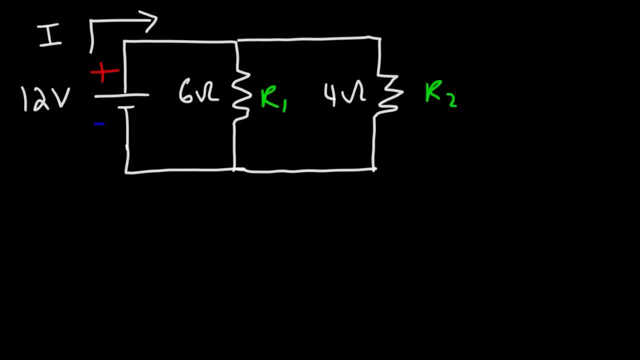 going to flow away from the battery. Feel free to pause the video and try this problem. Keep in mind this is conventional current, which is in the opposite direction of electron flow. So how can we determine the current flowing in a circuit? At this point, the current will split off into two directions. 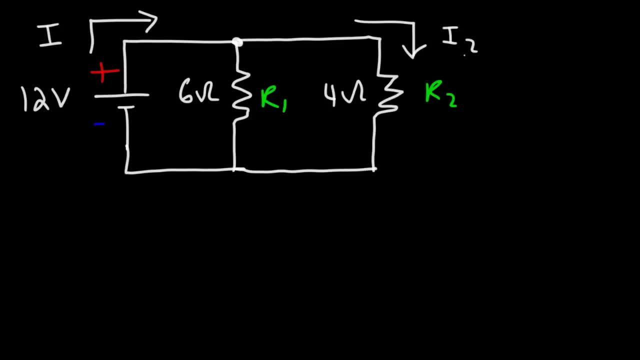 The current that flows through resistor 2, we're going to call it I2, and the current that flows through resistor 1, that's going to be I1.. The current flowing from the battery is the sum of I1 and I2.. So if we could find these, 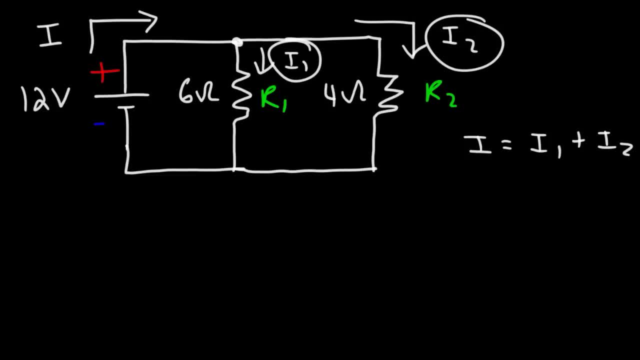 individual currents. if we can calculate the value of the current flowing from the battery, then we can determine the amount of current emanating from the battery. Now what we need to use is Ohm's Law. V is equal to IR. Now let's say, if we want to find I1, the current flowing through resistor 1.. We'll 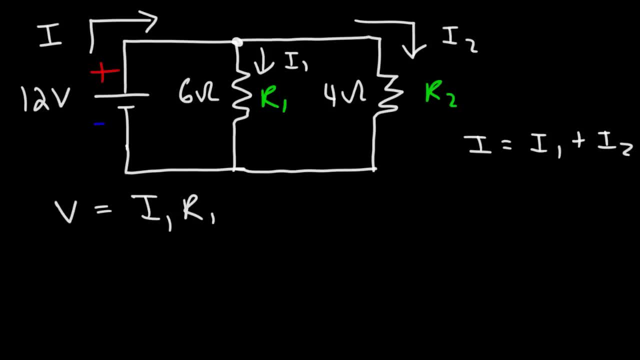 need the voltage across that resistor and the resistance itself. In a parallel circuit, the voltage across the resistors connected in parallel will be the same. Both resistors are connected across the same 12 volt battery. So V is 12 and R1 is 6.. 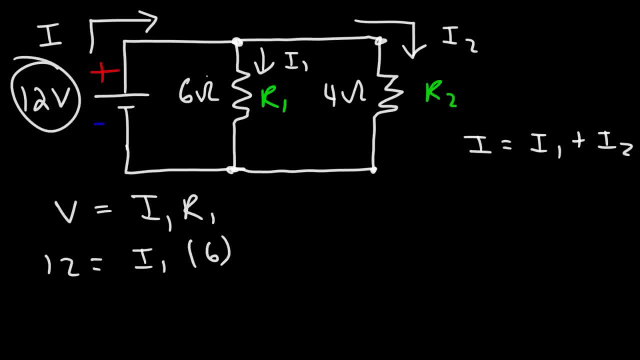 So I1 is simply the voltage of battery divided by the resistor, so it's 12 divided by 6.. So the current flowing through R1 is about 2 amps. Now lets' do the same for the other current, I2.. 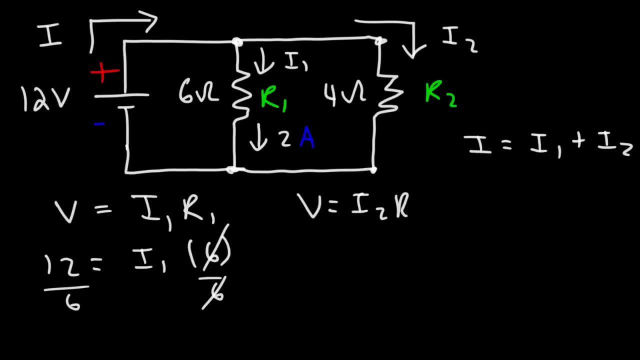 So V is equal to 2 volts. Now, in order for this to work, the extra current starting in the capacitor is about 5 volts to I2 times R2.. If we divide both sides by R2, I2 is basically V over R2.. So it's going to be 12. 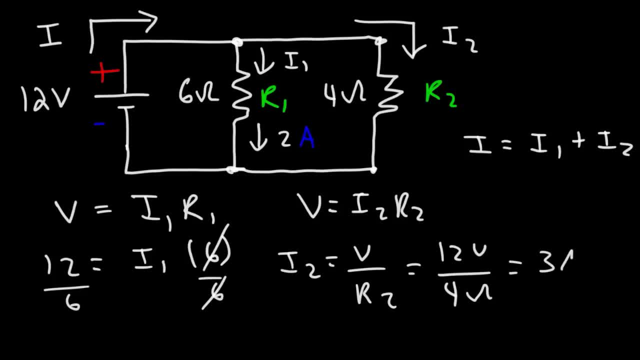 volts divided by 4 ohms, which will give us a current of 3 amps. So that is the current that is flowing through the second resistor. So now we can calculate the total current in the circuit. It's I1 plus I2.. So that's going to be 2 amps plus 3 amps, which is 5 amps. 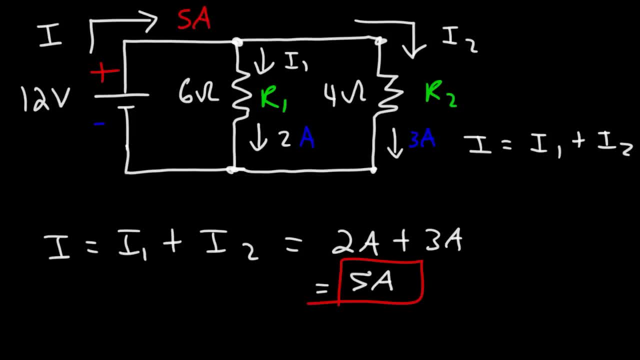 And so that's the amount of current that is flowing away from the battery. So that's one of the simplest ways in which you could determine the current flowing in a parallel circuit. Now let's work on another example, But this time we're going to have three resistors. 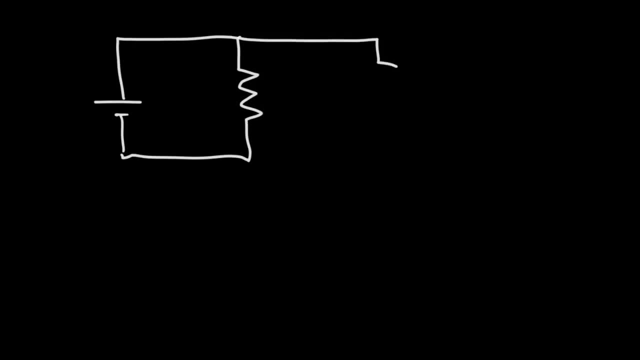 Connected in parallel with respect to each other, But the process for solving this circuit is the same as the other one. So let's name these resistors first. So we have R1, R2, and R3.. Let's say that the battery's voltage for this example is 30 volts. We're going to say that R1. 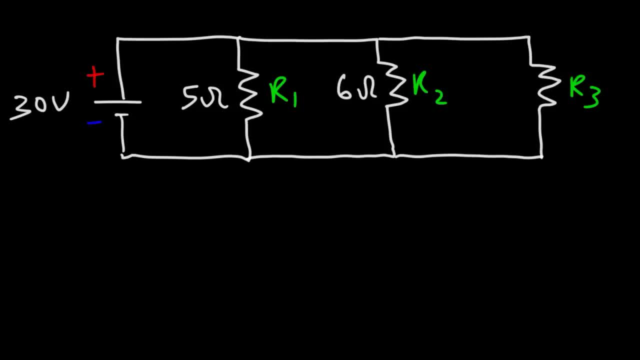 is 30 volts, So we're going to say that R1 is 30 volts. So we're going to say that R2 is 30 volts, R2 is 5 ohms, R2 6 ohms And R3 is going to be 10 ohms. So go ahead and calculate the current. 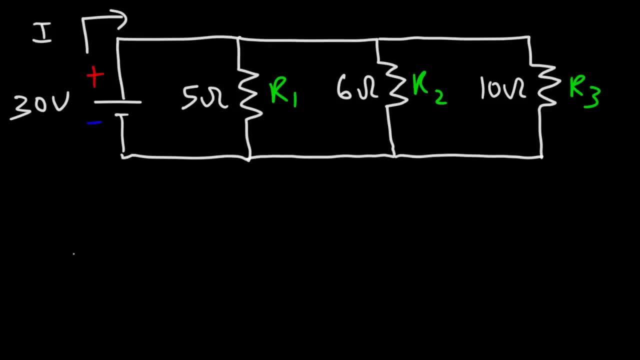 that is flowing in a circuit from the battery. So we need to calculate I1,, I2, and I3. So let's go ahead and do that. So we know that V is equal to I1 times R1. But we're going to use this version of that equation: I1 is V over R1.. V being 30. 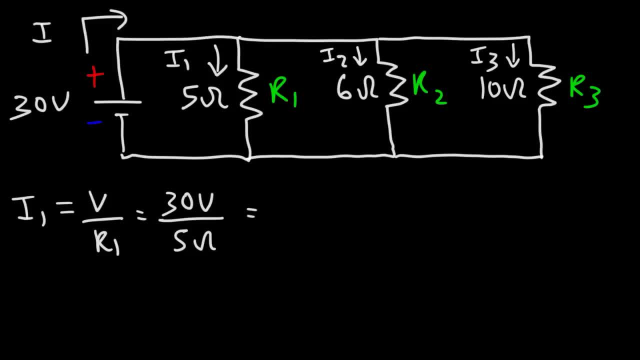 volts. R1 is 5 ohms, So 30 divided by 5. That will give us a current of 6 amps. I2 is going to be V over R2.. So V is the same. The 30 volt battery is connected across all three resistors, So any. 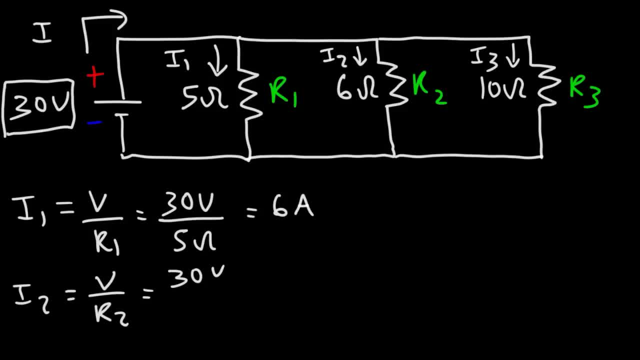 time you have a parallel circuit. the resistors in a parallel circuit all have the same voltage across them. R2 is 6 ohms. 30 divided by 6 is 5.. Now for I3.. Okay, that is a messed up looking. 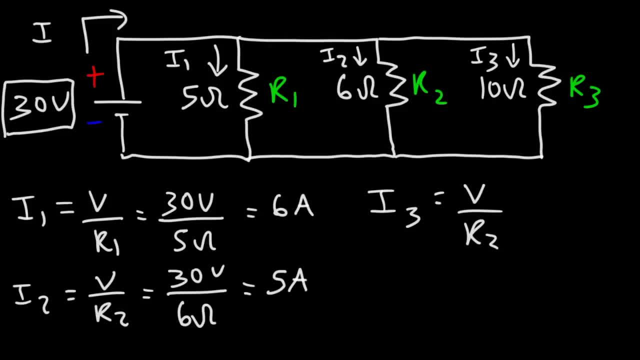 3.. Let's do that again. I3 is going to be V over R3.. So that's 30 volts divided by 10 ohms. So that's a current of 3 amps. So now that we have the current flowing through, 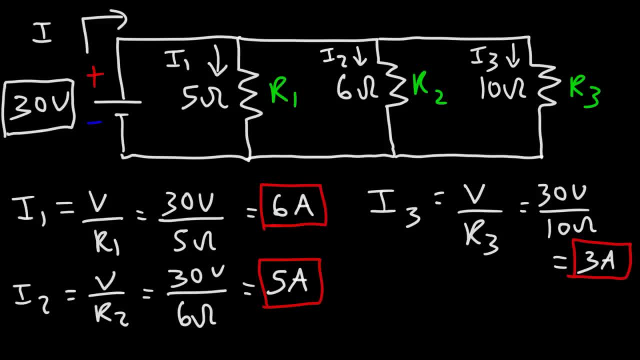 each resistor. we can now calculate the current leaving the battery, And that current is basically the sum of these other currents, I1,, I2, and I3.. So it's 6 plus 5, which is 11, plus 3,, which is 14.. So the current leaving the battery is equal to 14 amps. 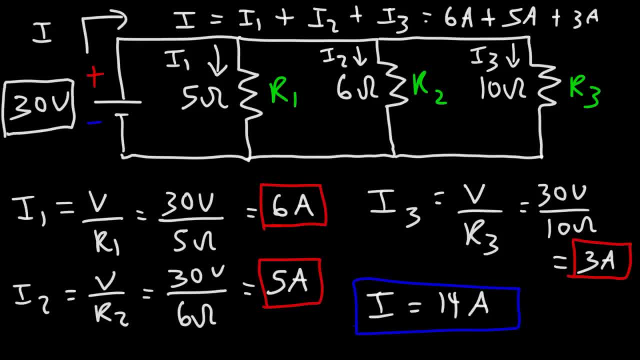 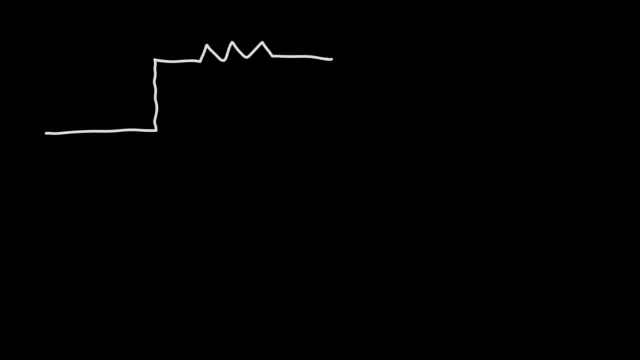 So that's a quick and simple way in which you can calculate the current flowing in a parallel circuit. Now let's work on a different type of example. So once again, we're going to have two resistors connected in parallel with respect to each other. 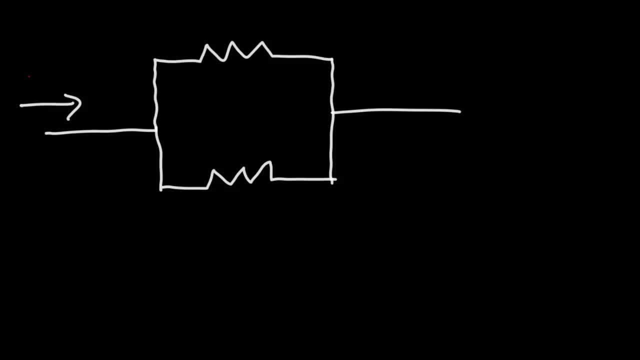 And let's say we have a current of 6 amps flowing at this point in a circuit. Let's call this R1 and R2.. And let's say that R1 has a value of 5 ohms And R2 has a value of 10 ohms. What is the current that is flowing? 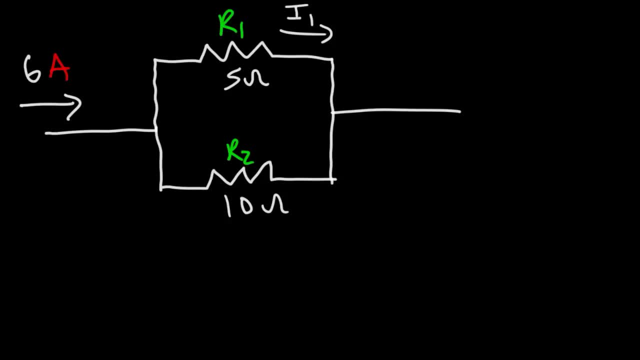 through resistor 1?. So what is I1 in a circuit? Feel free to pause the video and think of a way in which you can calculate I1.. You can do it conceptually or you can actually use a formula to get this answer. 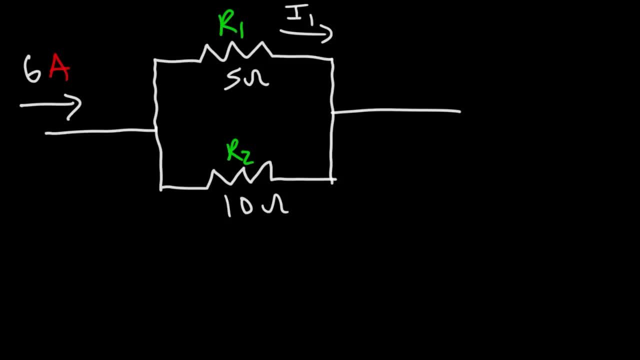 But see if you can figure it out. So let's begin. Let's think about it conceptually Now. R1 has a lower value than R2, which means that I1 should be greater than I2, because, as the resistance decreases, the current increases, given that the voltage is constant. 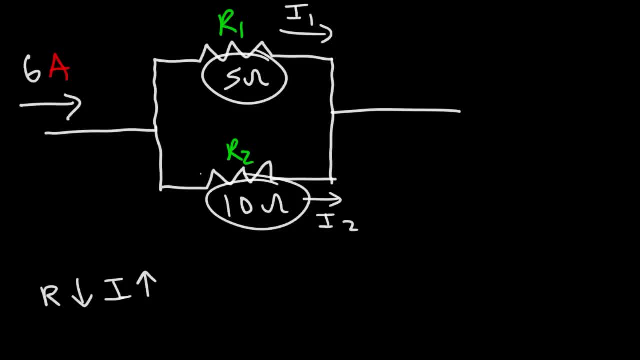 So notice that R1 is half the value of R2. That means that I1 must be greater than R2. And R2 must be twice the value of I2.. And let's call this IT the total current. The total current is the sum of I1 and I2.. 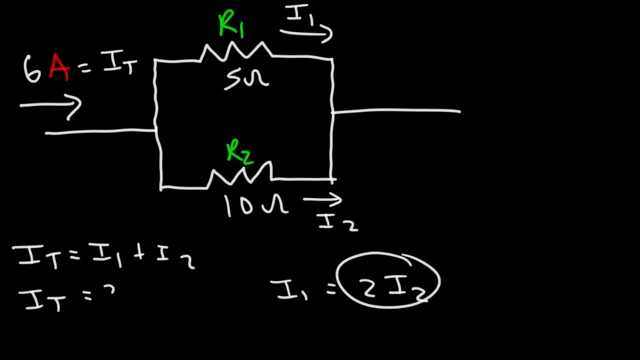 So replacing I1 with 2I2, we get this. So IT is 6, 2I2 plus 1I2 is 3I2.. And then 6 is 2I2.. And 6 divided by 3 is 2.. 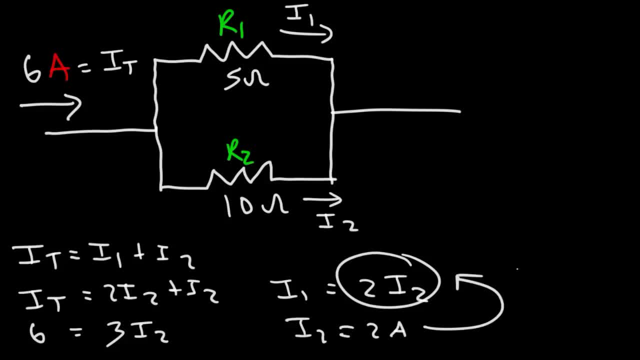 So I2 is 2 amps. Plugging it into this equation, 2 times I2, or 2 times 2, I1 is 4.. So that's a quick and simple way to get the answer for this problem. Now there's a formula that will help you to get that same answer. 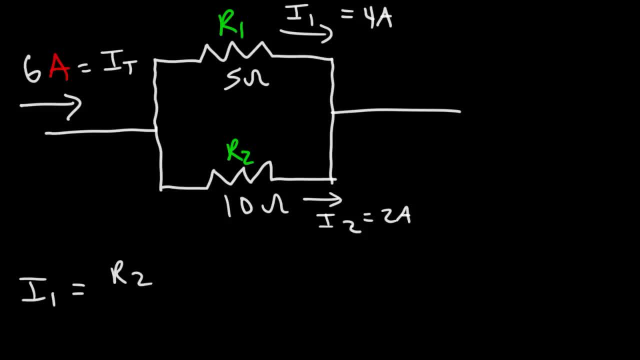 I1 is equal to R2 divided by R1 plus R2, times the total current. So R2 is 10,, R1 is 5, and then IT that's 6.. So 10 times 6 is 60,, 5 plus 10 is 15,. 60 divided by 15 is 4.. 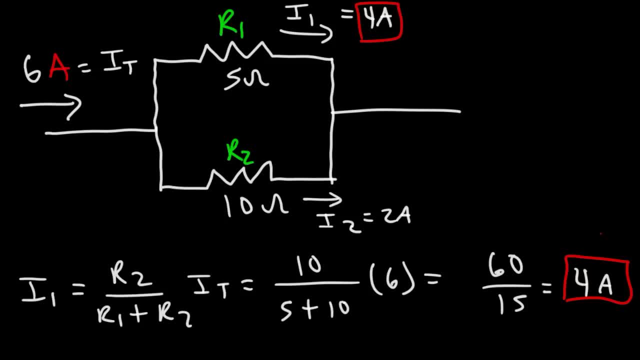 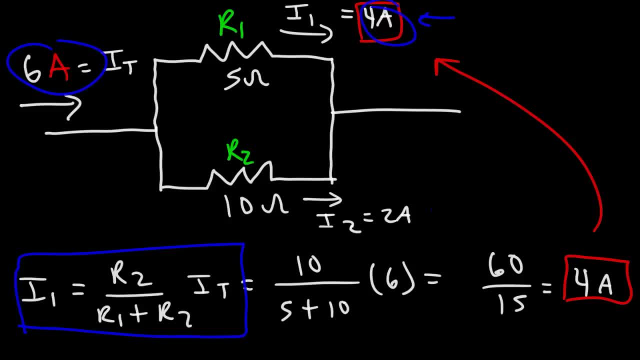 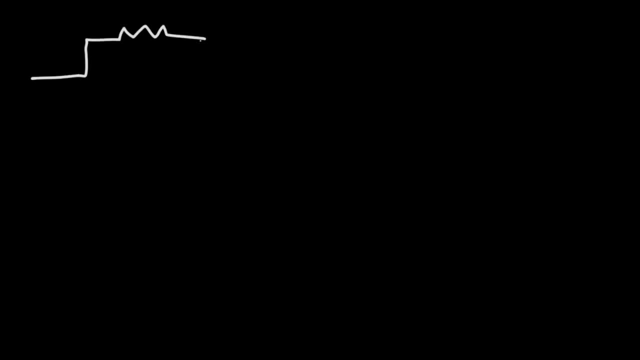 Okay, Okay, Once you have this answer, you could subtract these two values to get this answer: 6 minus 4 is 2.. Now let's talk about how we can derive the formula that we just used to get the answer. That is the second formula. 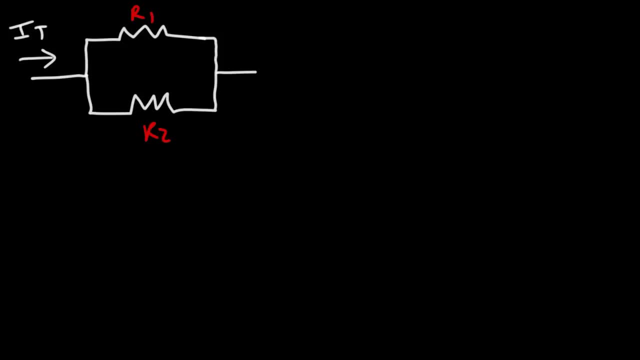 Now, as we said before, the voltage across two resistors in parallel is going to be the same. So the voltage across R1 is the same as the voltage across R2. And based on Ohm's law, we can say that V1 is I1 times R1, and V2 is I2 times R2.. 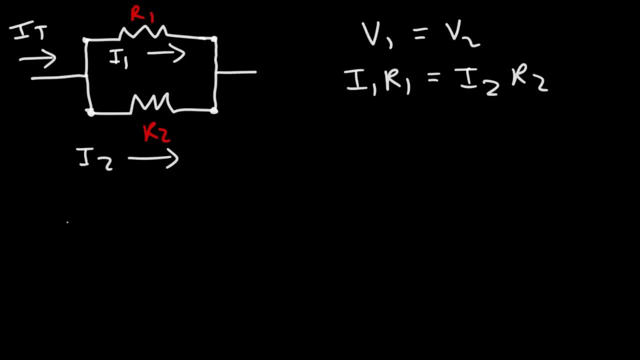 So here's I1,, here's I2.. And we know that IT is basically I1 plus I2.. So, solving for I2, We need to move this to the other side. So I2 is IT minus I1. So I'm going to replace I2 with this. 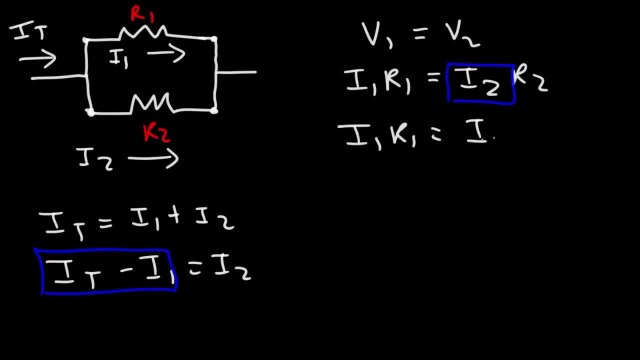 So I1 R1 is equal to the total current minus the current flowing through resistor, 1 times R2.. Now let's distribute R2.. So I have I1 R1. that's equal to IT times R2 minus I1 R2..